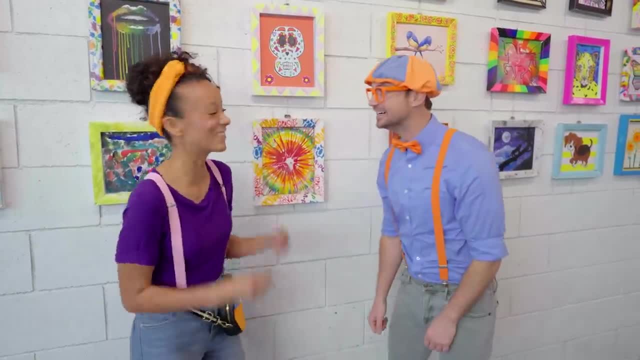 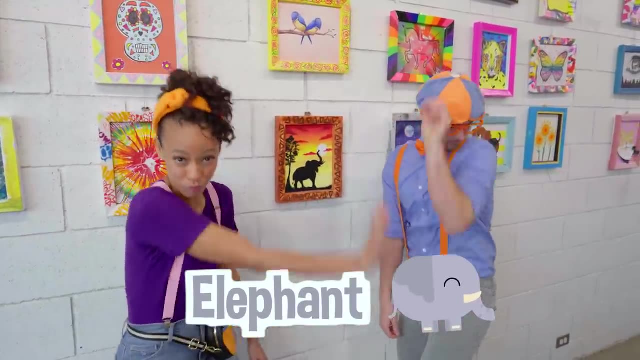 Oh, look at this one. Whoa, It's kind of spooky. Yeah, I love the teeth. Oh, and look an animal. Oh, And an elephant. Yeah, Wow, That's so cool. and look at the two little birds. 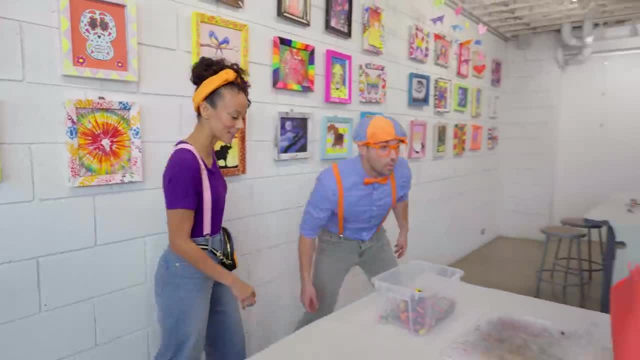 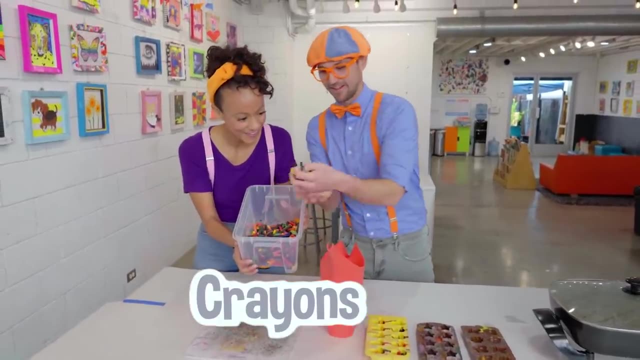 Tweet-tweet. Whoa, Mika, check it out. Ooh, what's on this table? Whoa, Looks like a lot of cool things. Yeah, oh, look Crayons. Whoa, so colorful, So many different crayons. 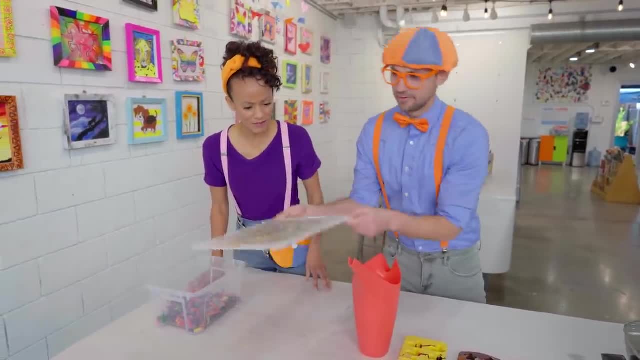 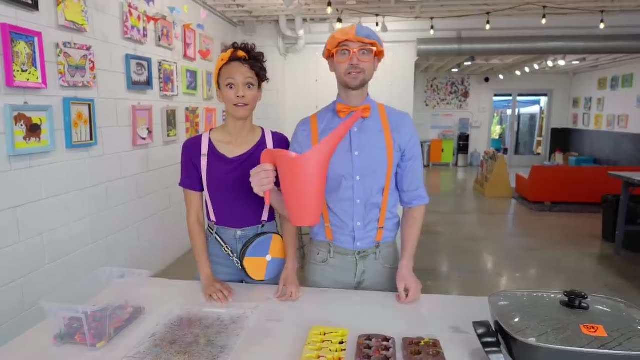 Mm-hmm, Whoa, look at this, a cutting board, What You usually find that in a kitchen. Yeah, I know, Interesting, Huh. And what's in there? Huh, looks like one of those things that you use to water plants with. 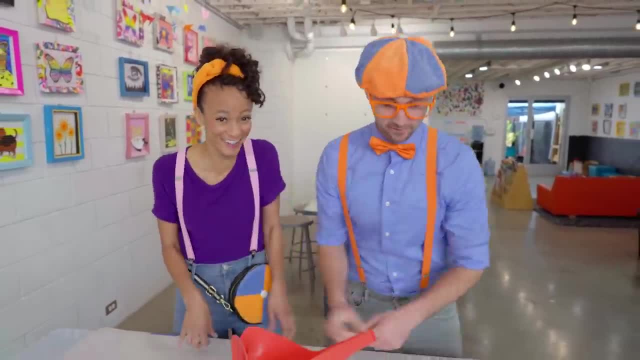 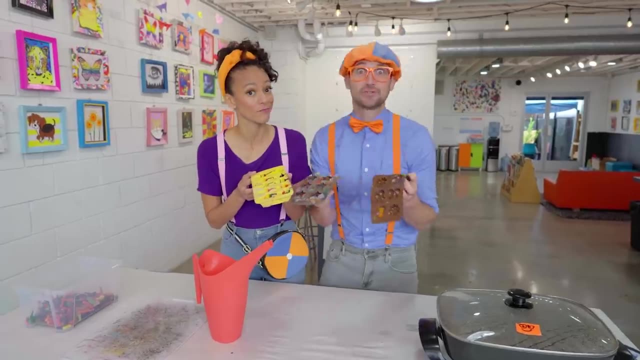 Yeah, there's water in there. Oh yeah, probably shouldn't pour that out. Whoa, look at these Molds- Something else you might find in a kitchen. Yeah, you could even put chocolate in these. Ooh, yummy. 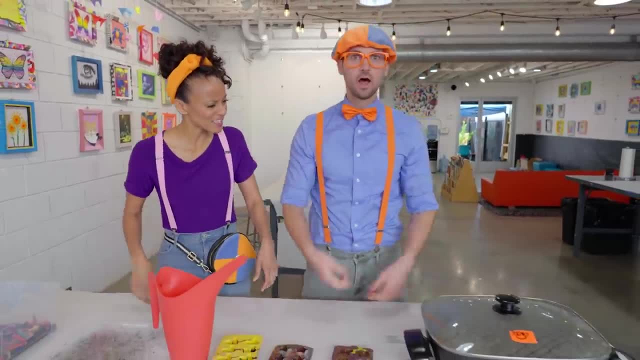 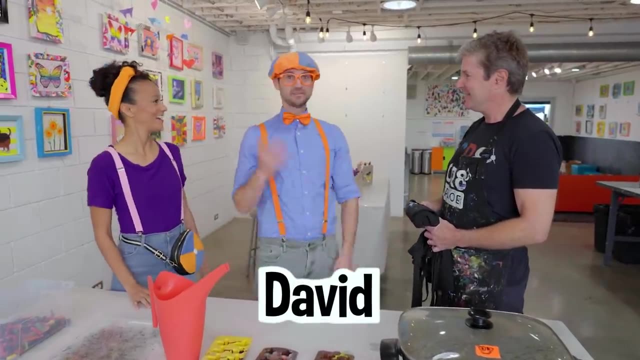 Whoa, hey, and a skillet Whoa. We must be cooking today. Yeah, cooking art, Hi, Oh hey, who are you? I'm David. Whoa, nice to meet you, David. I'm Blippi. 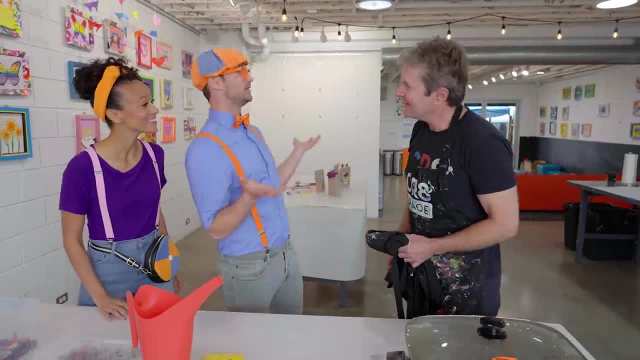 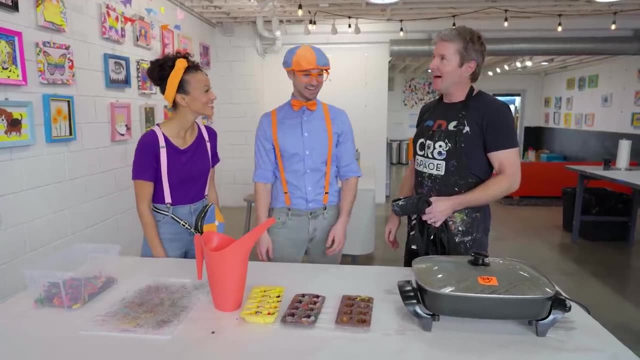 Hi Blippi, I'm Mika Hi, Mika Hi, What do you do here? Well, this is my art studio. Wow cool. We love it here. Yeah, It's really cool. Thank you, Yeah. 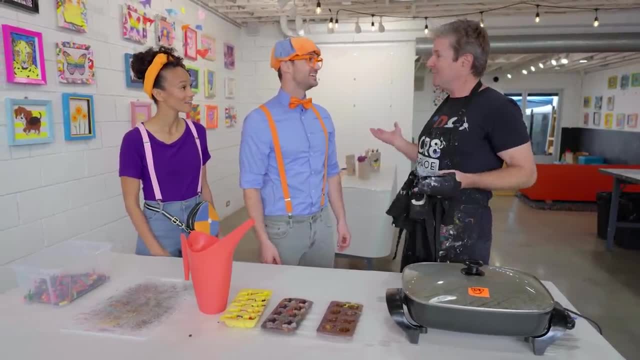 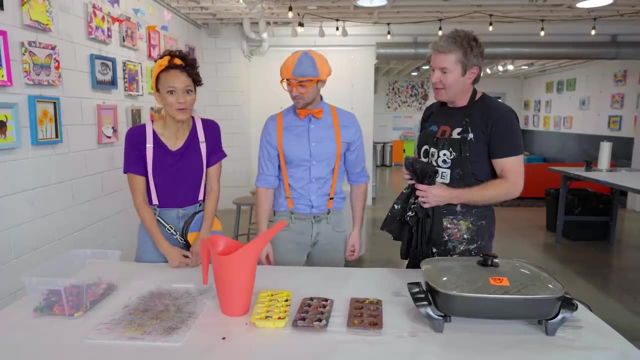 It's been a dream of mine to do this forever, and my dream came true. That's amazing. Yeah, whoa, I would love for you guys to try a little project with us today. Ooh, that's fun, That's fun. 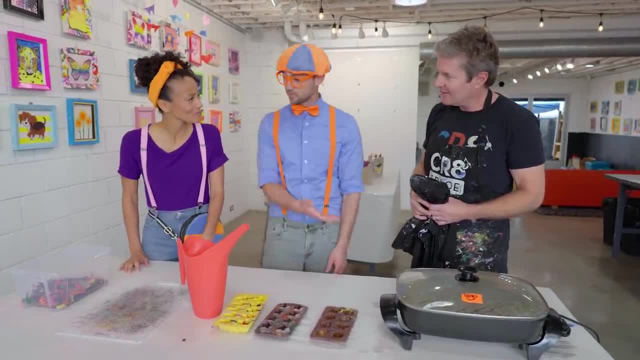 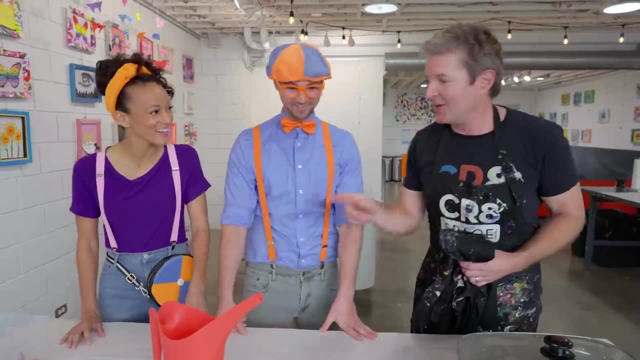 Do you know what all this stuff is for? No, we couldn't figure it out, but we saw everything that was here. Yeah, Well, it looks like we're going to cook. Yeah, it does Surprise, We're going to cook crayons. 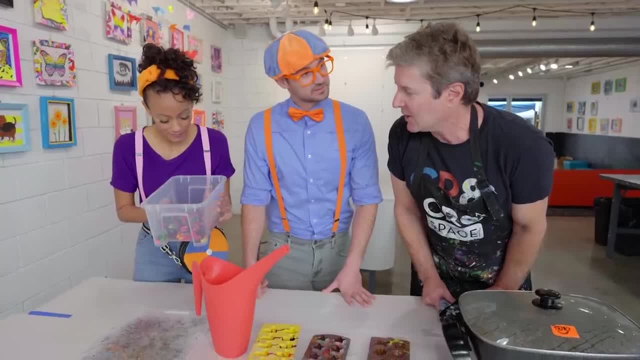 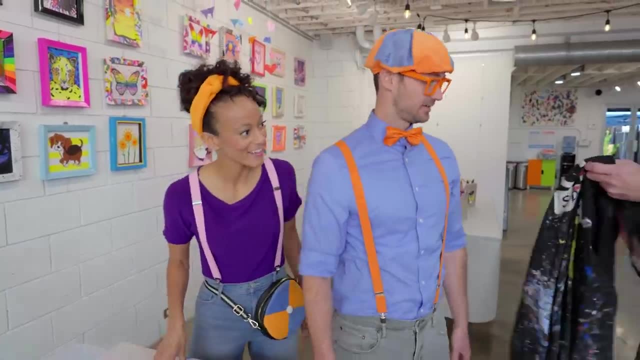 Cooking crayons. You can't eat crayons, So these crayons are going to be reused. We're going to turn them from something old to something new. Oh crazy, Cool. How are we going to do that? Let's get started. 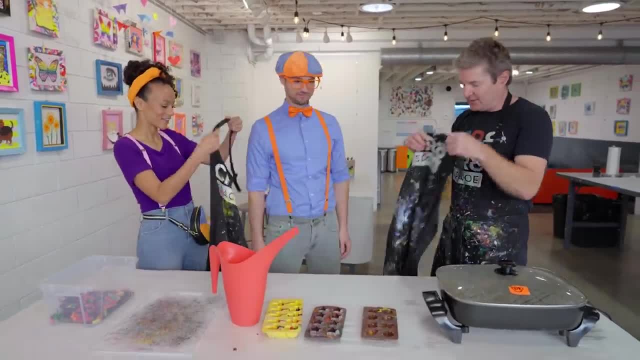 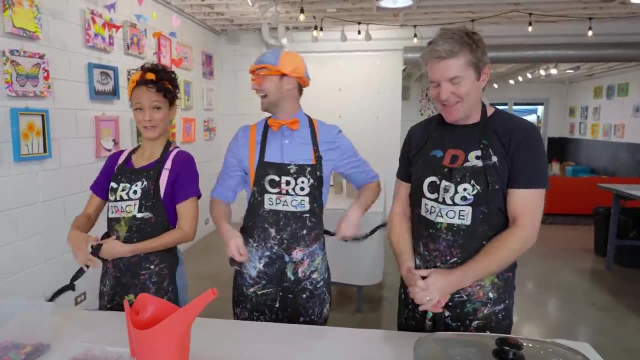 OK, First of all, here, Here you go. These are our aprons. Thank you, You can put them on to keep your cool clothes nice and clean. Oh great, Thank you for saying that we look so cool. Oh yeah, thanks, Selma. 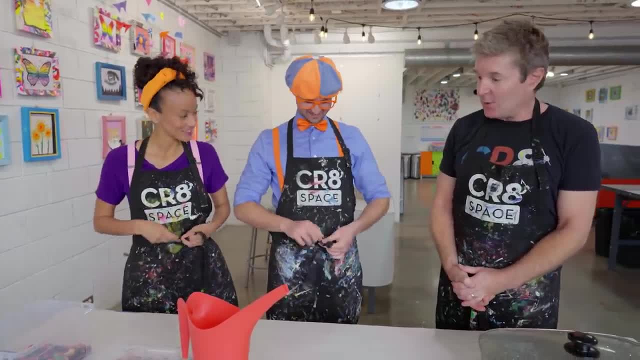 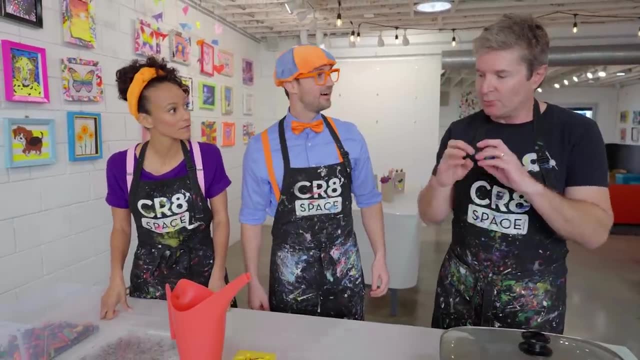 We try every day. OK, So we're going to pour water into this skillet. It's going to get hot And while it's heating up, we're going to take those crayons and break them into pieces. OK, Sprinkle them in the molds. 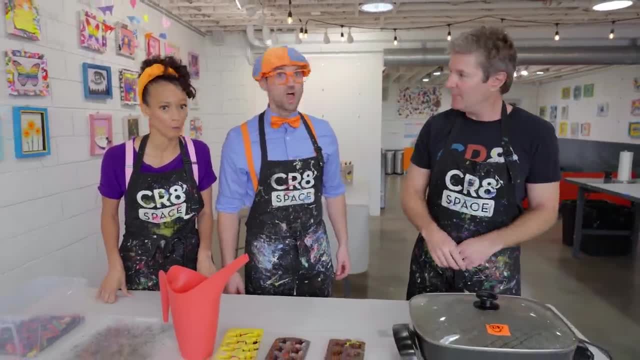 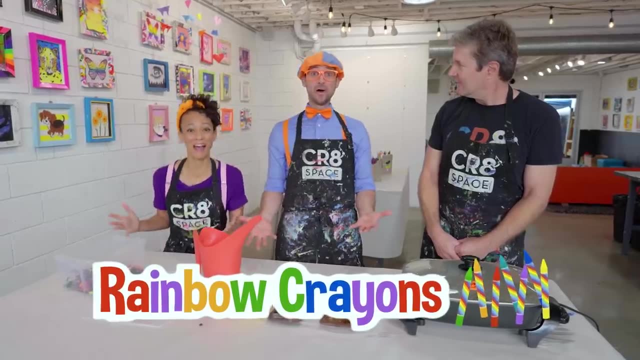 Put the molds into here And then we're going to cook them. So we're going to mix these crayons together. They're going to melt, We're going to put them in there And then we're going to make rainbow crayons. 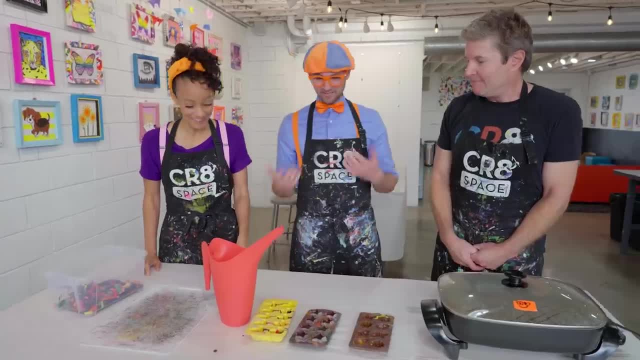 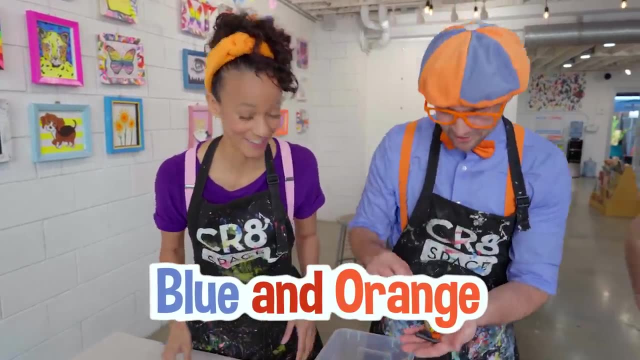 Rainbow crayons, Rainbow crayons. Yeah, Love it Well, shall we? Yeah, Sure, All right, Pick your favorite colors. OK, All right, Little lippy Ooh, let's see. Well, I like blue and orange. 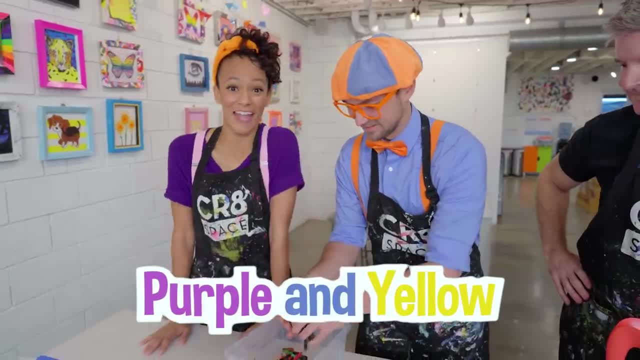 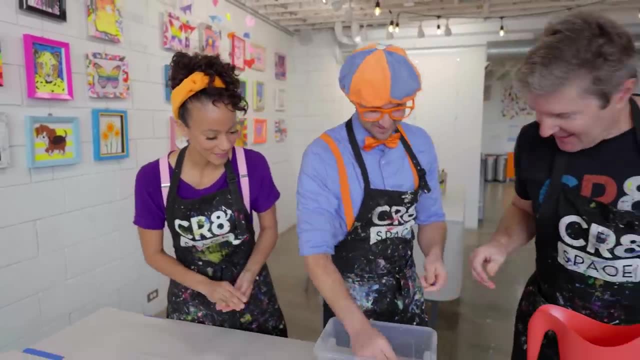 Oh yeah, he really does. OK, And I love purple and yellow. Yeah, Check it out. Blue and orange- Ooh, there's some yellow there. I like orange and orange. Orange and orange- Yeah, Oh, here you go. 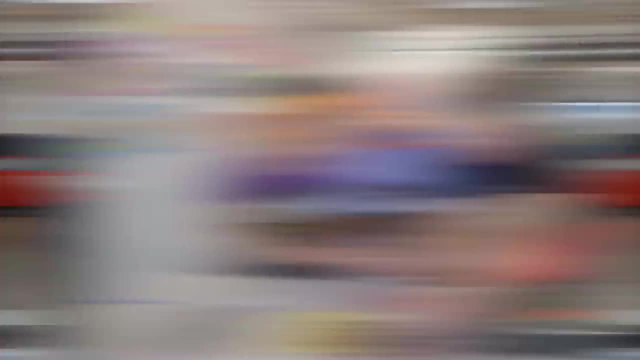 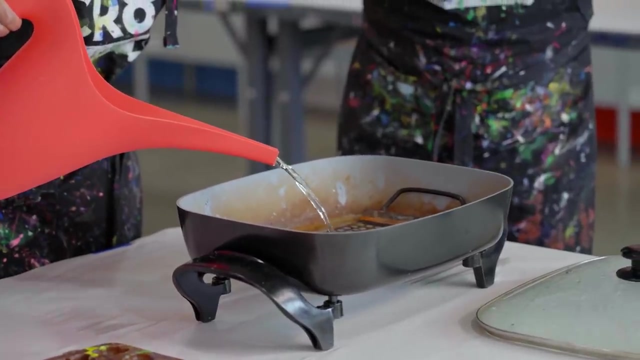 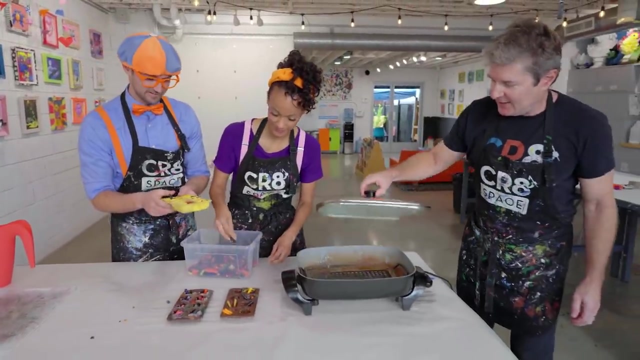 Thank you, OK, And then we'll break them in there. OK, OK, you ready? Yeah, Can we put it in there now? Yeah, All right, So go ahead, and if you don't mind, it's going to get hot, so just be really careful. 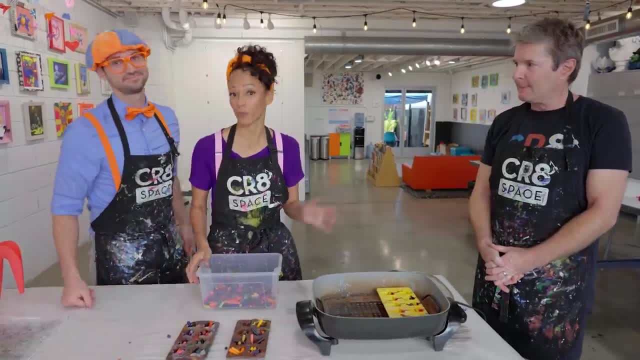 OK, Good job. All right, If something gets this hot, it's a good idea to do it with a grown-up. Yeah, Yeah, All right. and here's another one That looks great. Just set it right in the water. 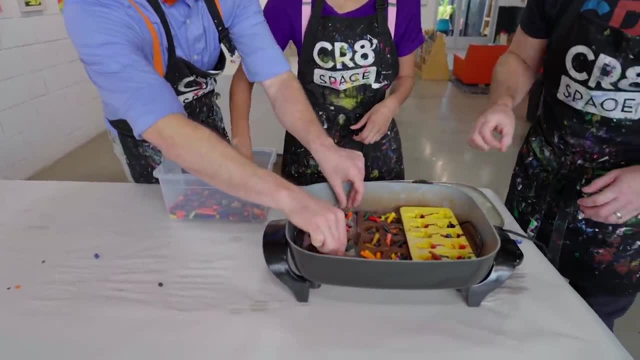 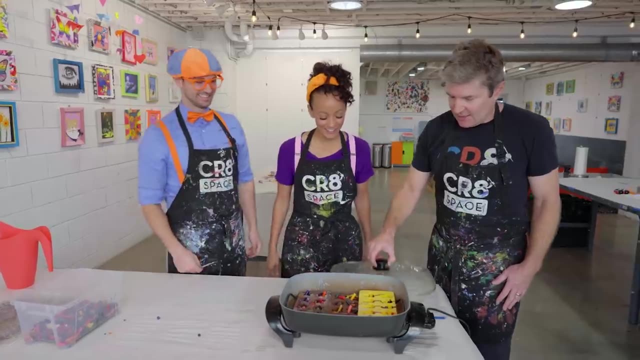 OK, And then make a little bend here. How about this one? Perfect, Wow. Oh you guys, these are going to be so cool. I'm so excited. Nice work, Thank you, I love your colors. Thanks, If you guys don't mind, I'm going to stay here. 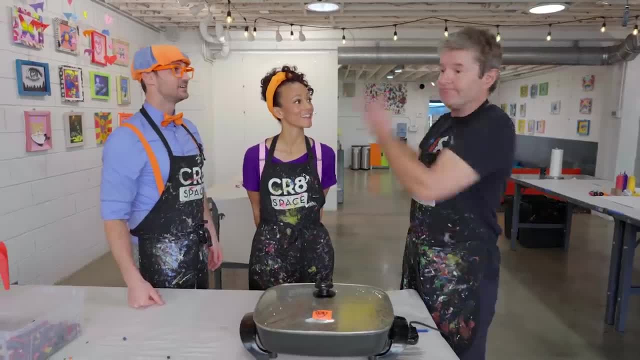 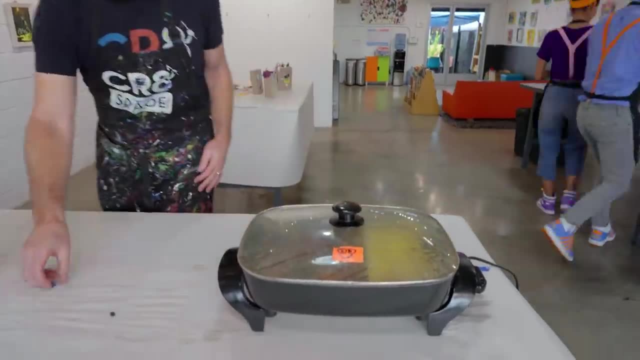 and watch this cook, OK, And if you want go and explore the art studio, All right. That sounds like fun, OK, Yeah, thanks, so much. Bye, guys, Have fun. Wow, Whoa, look at this place. 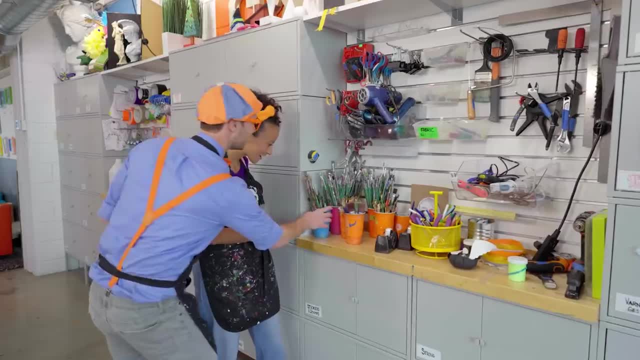 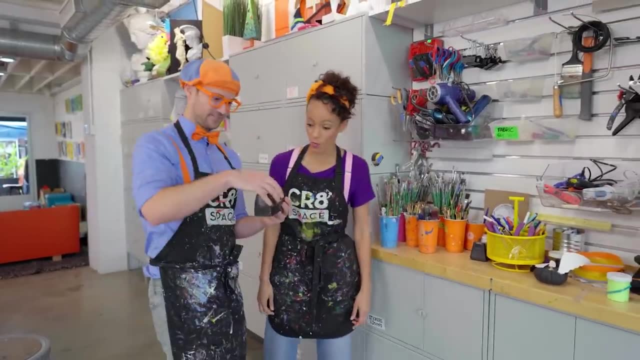 Yeah, Wow, Oh. look at all these scissors, Whoa, Oh. and look Paintbrushes, Yeah, a lot of paintbrushes. Wow, Sizes, Yeah, Oh. and some tape, Oh, Oh. Stick things together. 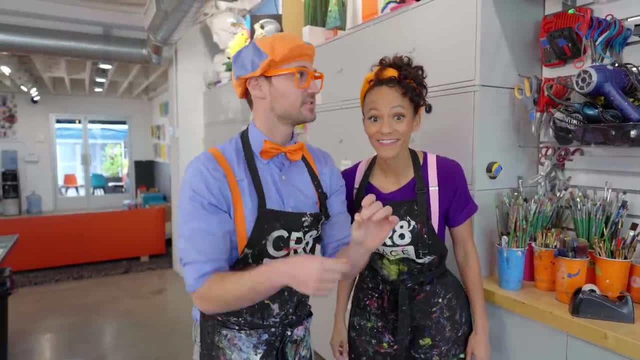 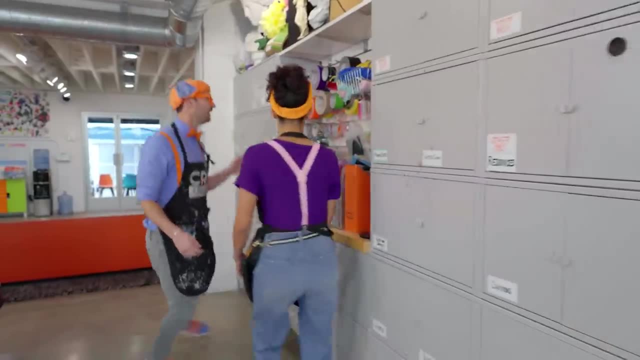 Oh Yeah, It's really cool how there's a lot of different materials to use for art. That's right, Oh, Oh, And there's even more over here. Whoa, Oh, check it out. More tape, Oh, some blue tape. 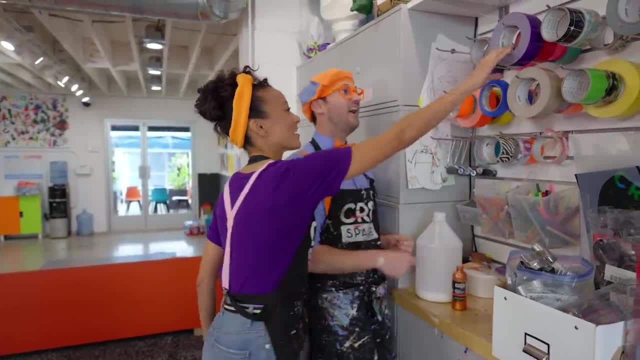 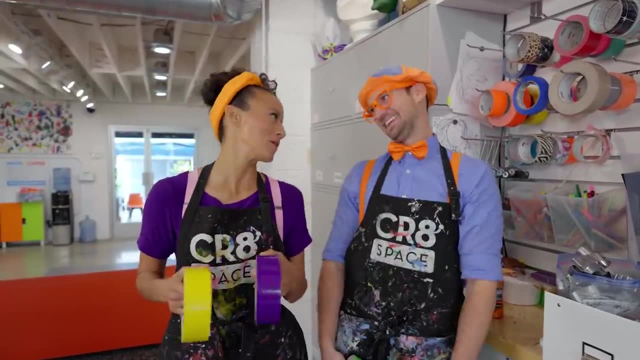 One of my two favorite colors. Yeah, Whoa, Oh and look. Purple tape, My favorite color. Yeah And look, Mika. My other favorite color, You know me so well- Yellow. Wow, this is so cool. 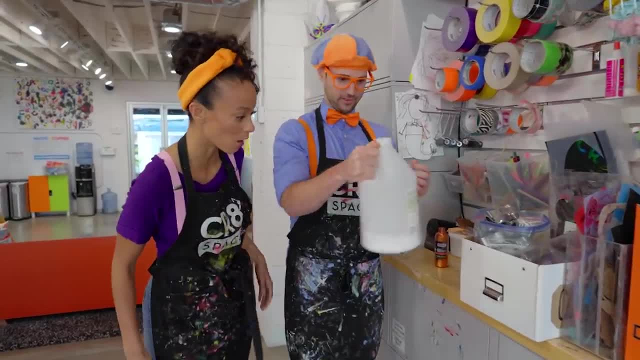 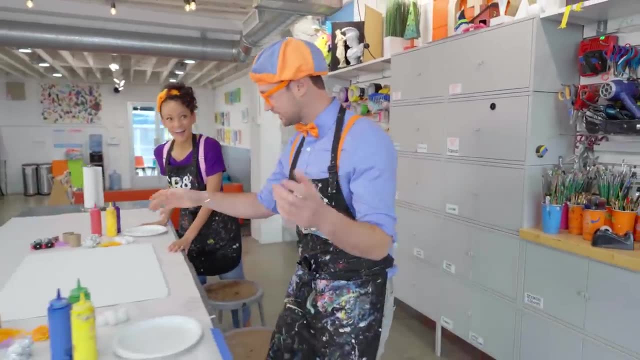 Whew, It looks like we have a bunch of glue. Whoa, that's a lot. Wow, Whoa, Mika, Check it out. Yeah, Whoa, look at all of this stuff. It looks like it's all set up for us to make a picture together. 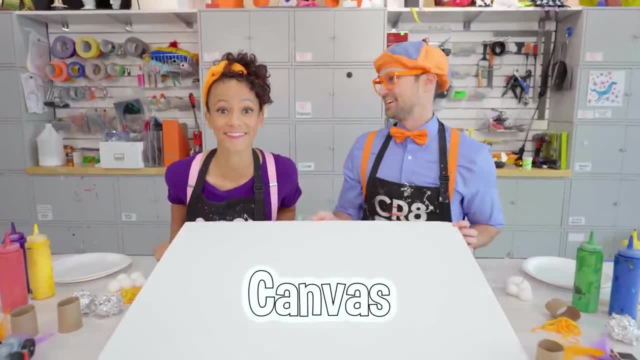 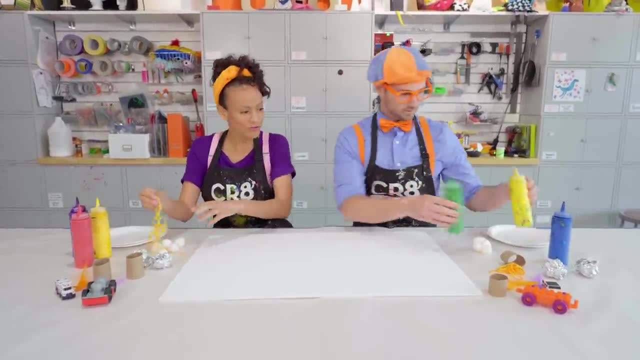 Yeah, check it out, This is our canvas. Mm-hmm. Should we make a picture together as a team? Yes, Okay, we have paint and paint. Oh yeah, Cotton balls- Green. Wait, some feathers. Where's the paintbrushes? 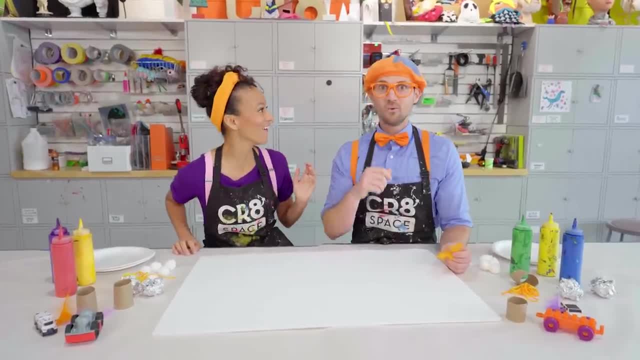 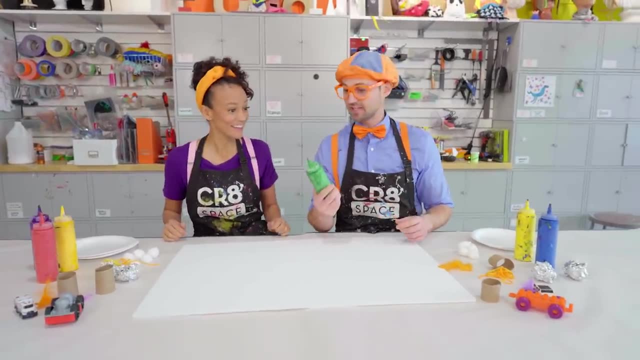 There's nothing on the table. I know What. We use these things: to get the paint onto the canvas. Oh yeah, you're right. So you're basically saying we can use, say this green, and then put it on this cardboard and then smash it down. 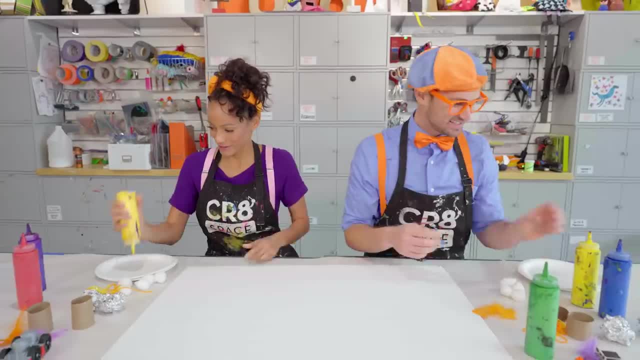 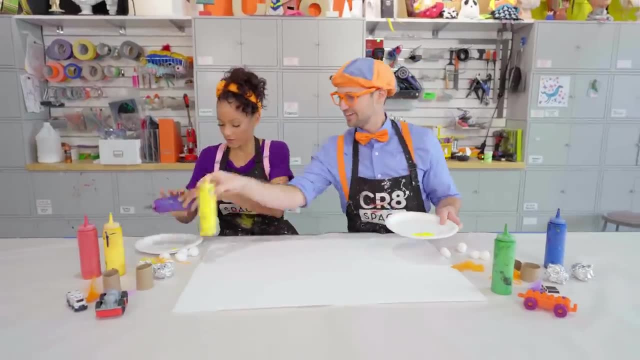 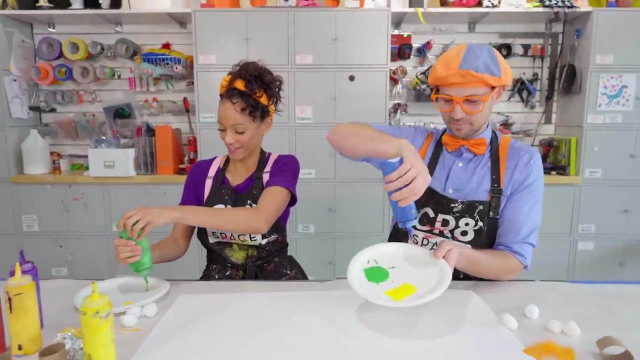 Oh yeah, Let's try, All right, yeah, Okay, Okay, let's see Yellow. I'm going to start with a yellow, All right, And here's some blue. Greg, what are you going to use first? 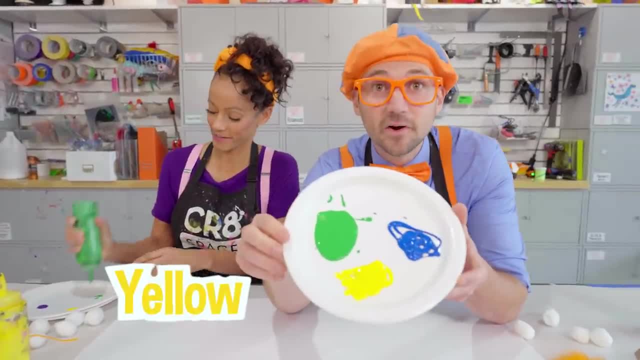 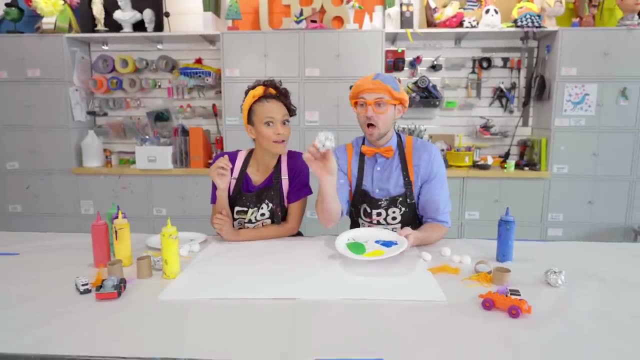 Let's see. Well, I have yellow, green and blue. Okay, I'm going to use some blue and I'm going to use some aluminum foil. What's it going to look like? All right, let's see. All right. 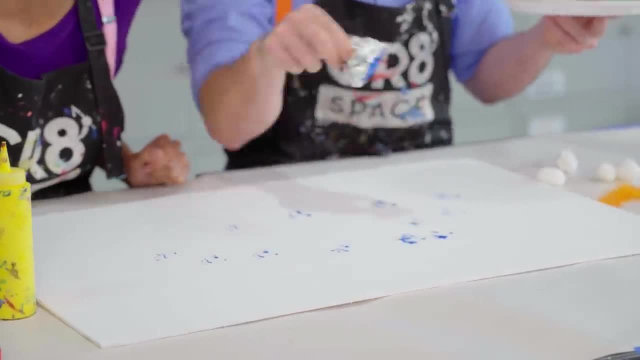 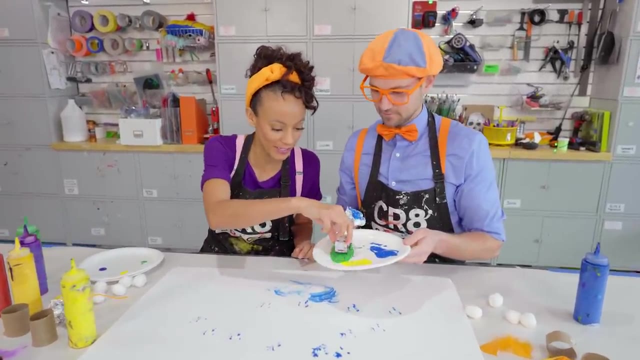 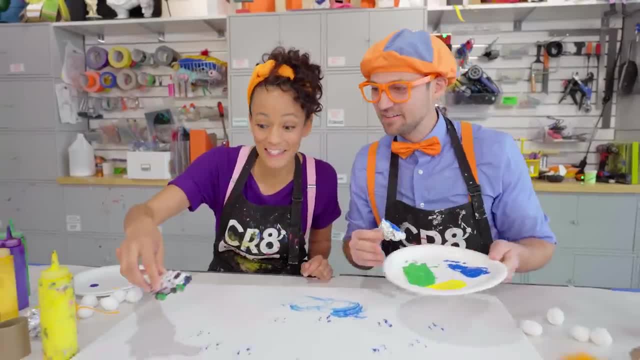 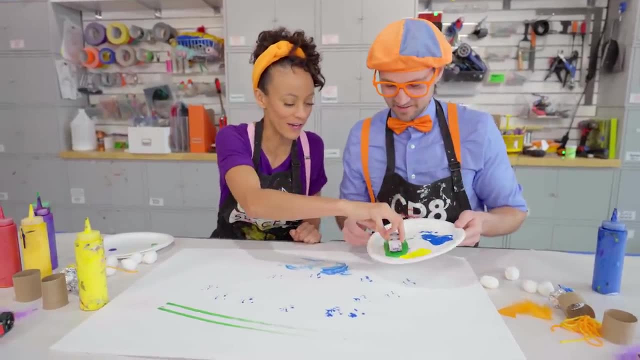 Thank you, Blippi. Oh, you're welcome. Whoa, All right, Let's see what it looks like. Speed painting: Whoa, Yeah, That looks cool. Wow, yeah, Get some more on there. Looks like some mud tracks. 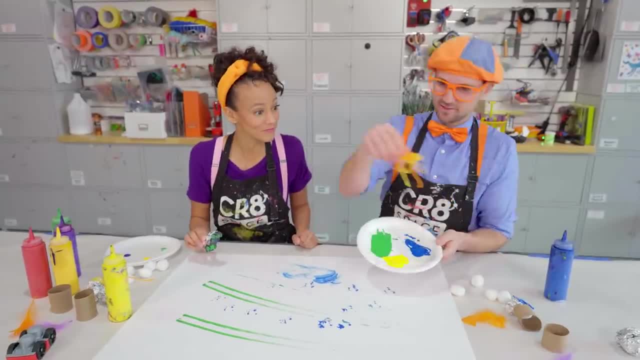 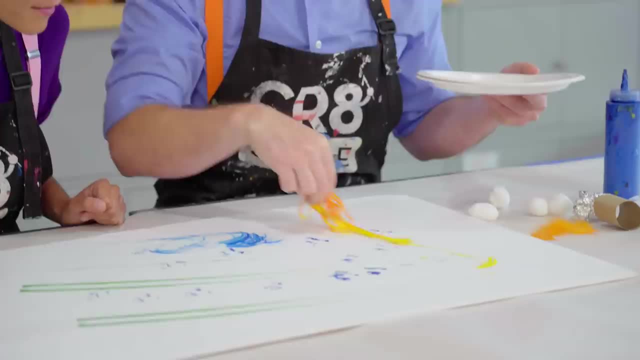 Yeah, You want to try? Oh sure, Oh, I'm going to use some yarn. Whoa, That's going to look silly. Yeah, Oh, okay, Here we go. Whoa, Whoa. Now, this is a masterpiece. 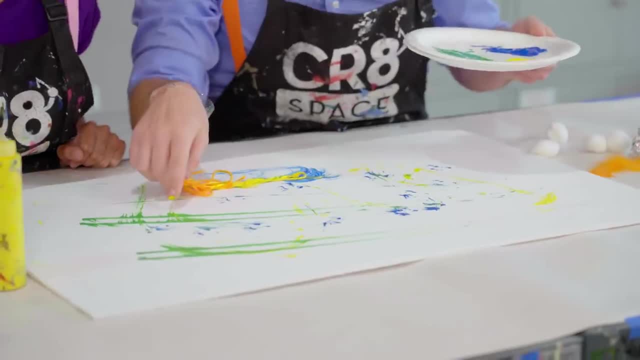 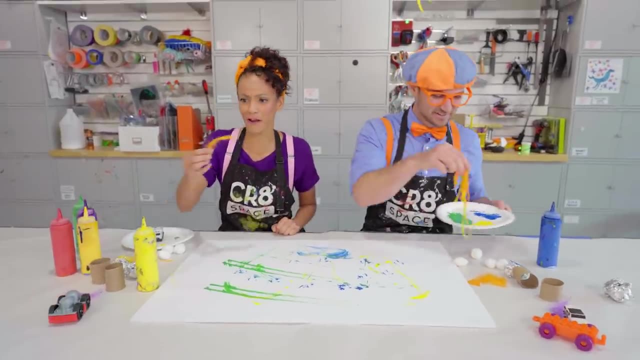 It sure is, Whoa. Look, It went over the wet paint, Yeah, And it looks like the vehicle is sliding around, slipping and sliding. Yeah, Ooh, I wonder what a feather would look like. Ooh, You want to try some. 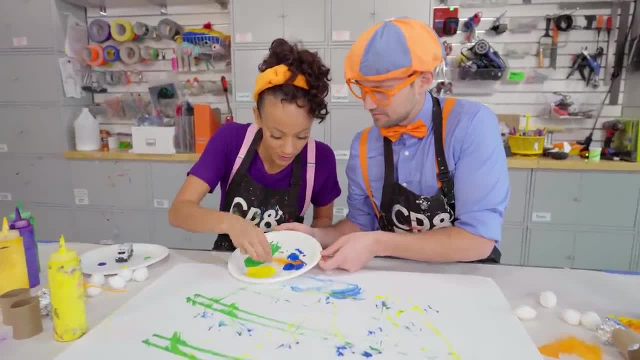 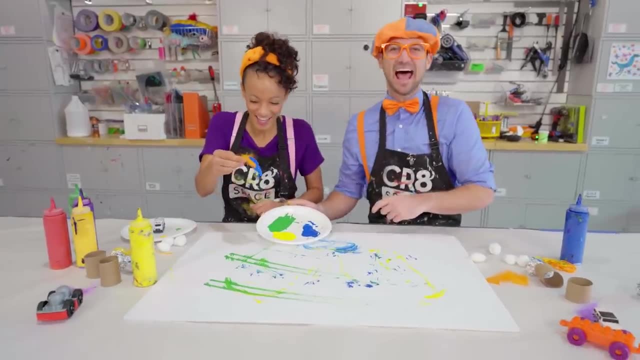 I'm trying some blue here. Whoa, Okay, A blue. What Blue? Whoa, Now, that's my kind of bird, All right, All right, Let's see. Okay, Whoa, Ooh, That looks so pretty Mika. 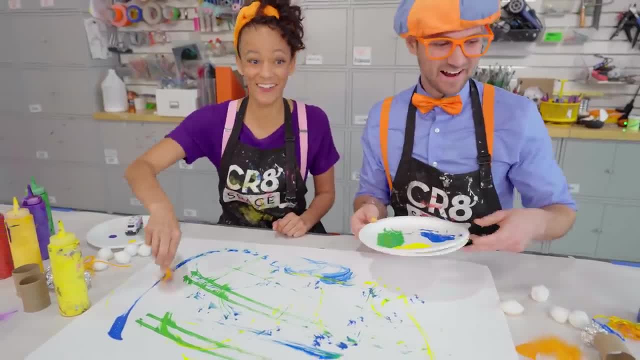 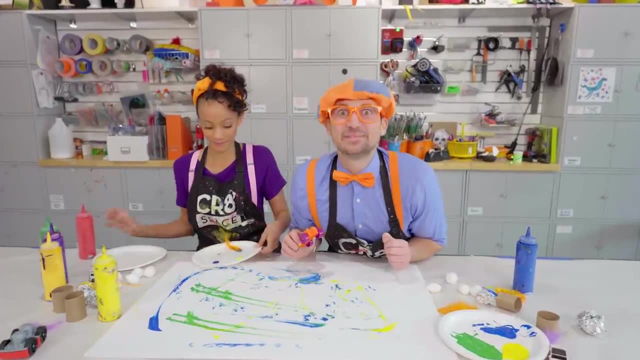 Thank you. Wow, Ooh, I have an idea. Do you think that red works? Let's try it. All right. Okay, This is going to be so silly. Okay, It works. Wow, It works really well, All right. 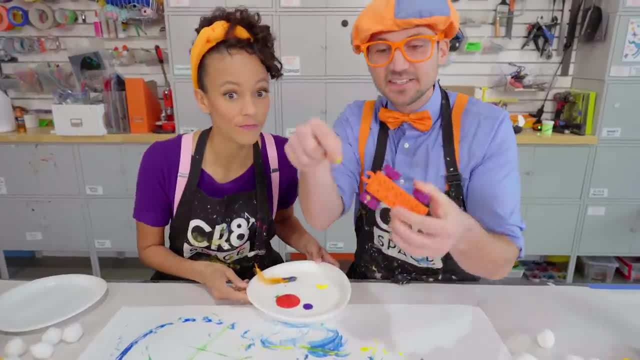 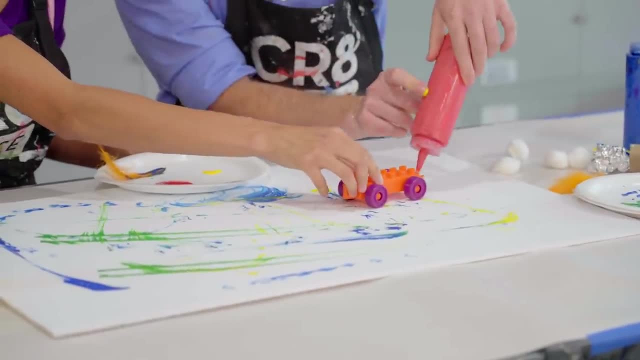 I'm going to need your help for this one. Okay, Okay, You see this. Yeah, Okay, Will you pass me the red? Sure? Okay, Okay, Ready Go, Whoa, Yeah, Whoa Cool, Very cool. 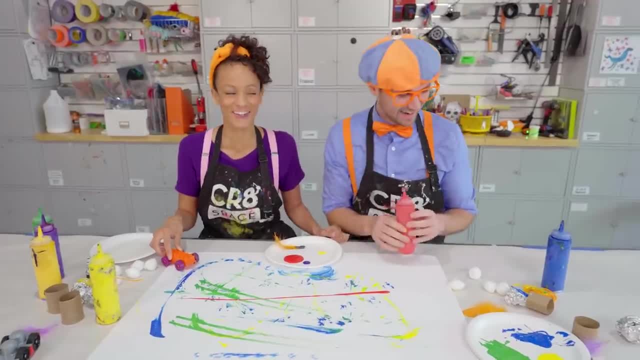 Good idea, Blippi. Oh, thank you so much. Now I want to put the wheels through the red here. Whoa Ooh and some cotton balls. All right, I'm going to mix all the colors together, All right. 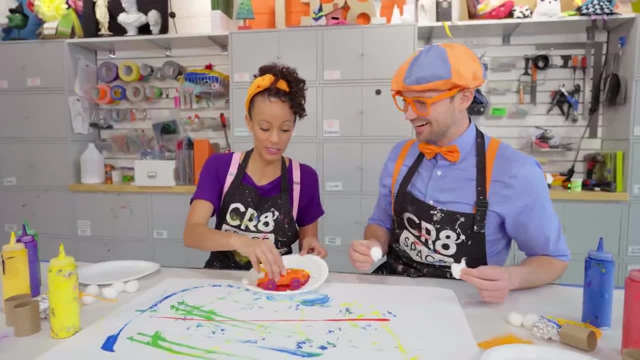 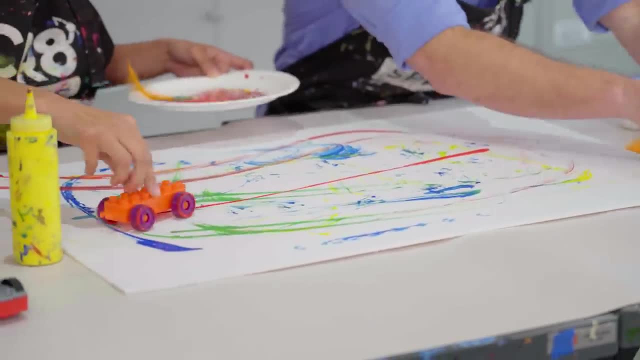 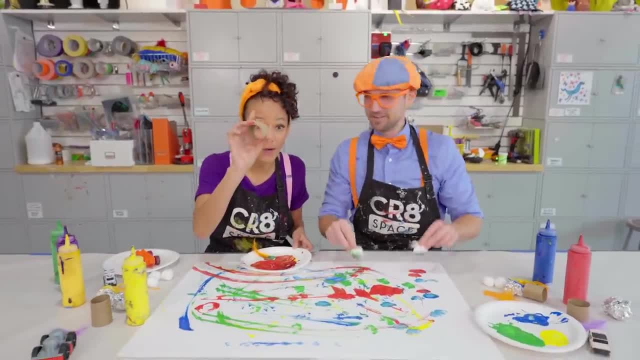 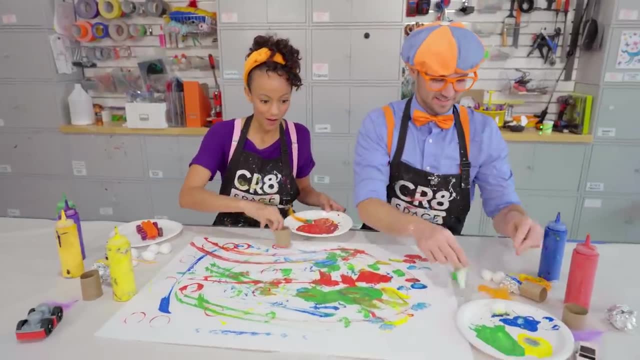 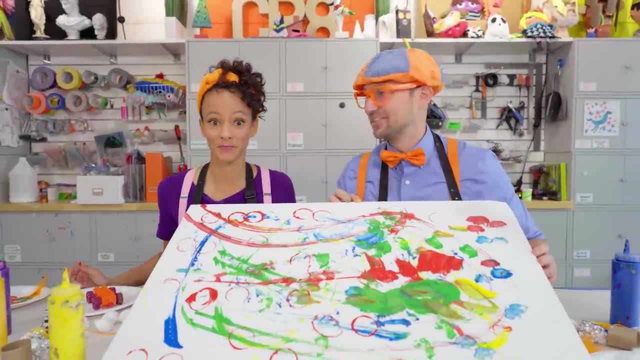 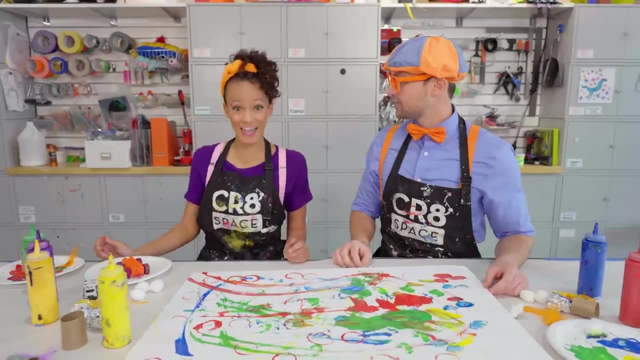 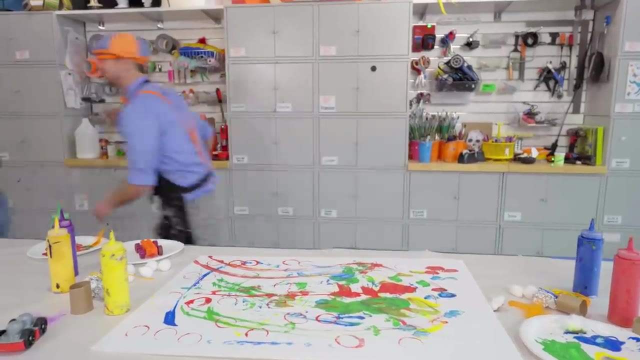 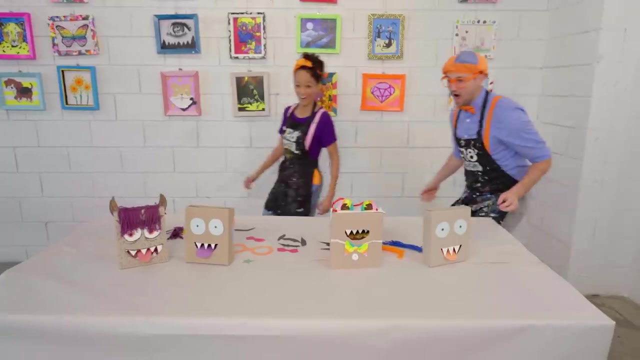 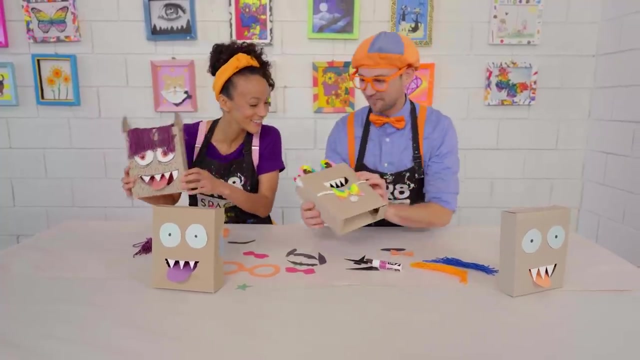 Yeah, Whoa, Look at the circles. Whoa. Well, Oh, Here we go. All right, Whoa, stay right here to dry. yeah, let's go find something else to do. okay, here you go. looks like box monsters, whoa, they're so silly looking. oh yeah, whoa, look, the eyes are on top. 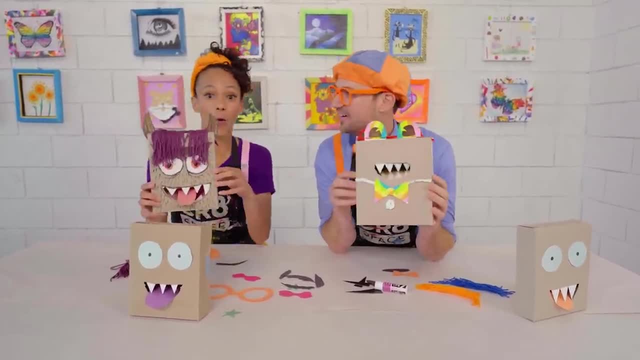 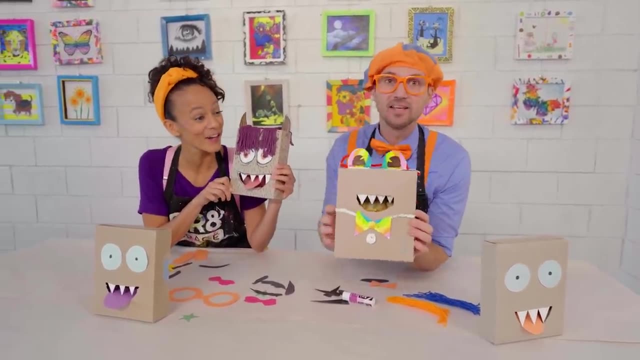 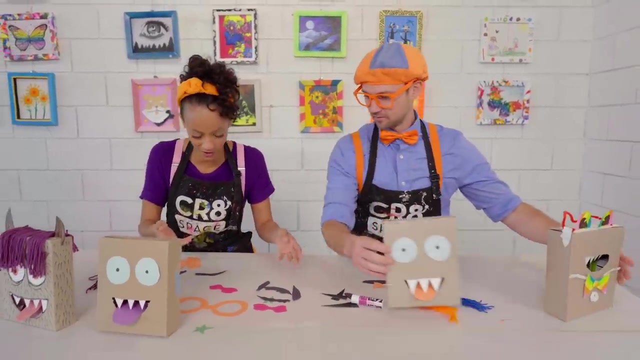 of the head- whoa, and look, this one has horns- whoa, and sharp teeth. oh. and this one has rainbow eyes and a bow tie, just like me. hey, that's right button, rainbow colors and blimpy. it looks like there's other bow ties and things here. oh, and some blank monsters. 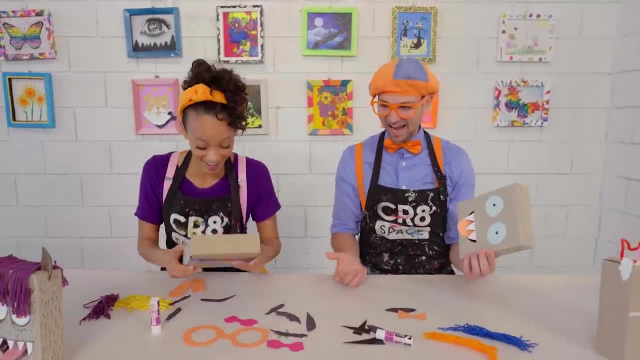 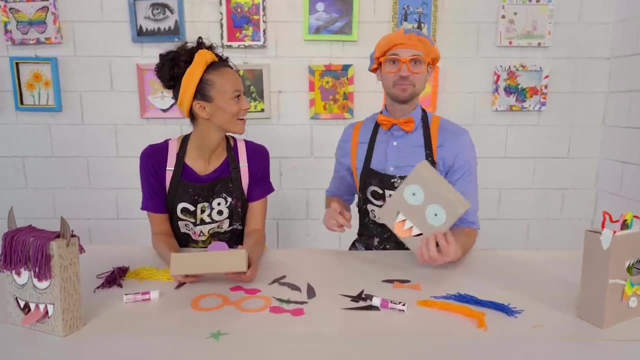 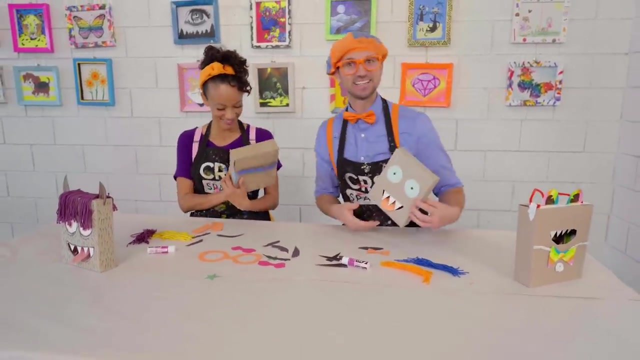 we can make our own monsters, yeah, oh, what kind of monster should we make? hmm, i know what i'm gonna make. what i'm gonna make: a blimpy monster box. oh, that's a great idea. i'll make a mica box- oh, that's a great idea too. whoa, look these, look like my glasses, oh that's. 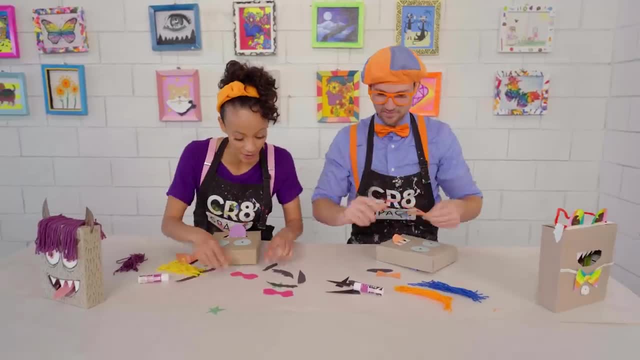 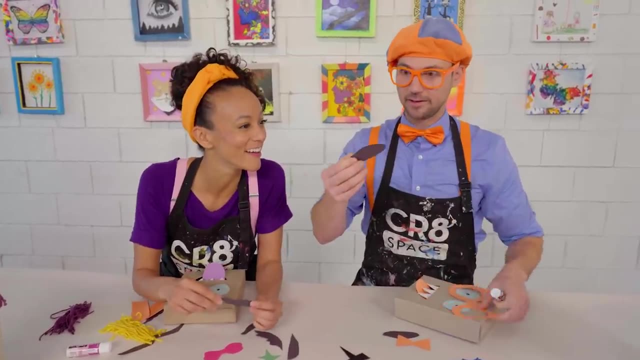 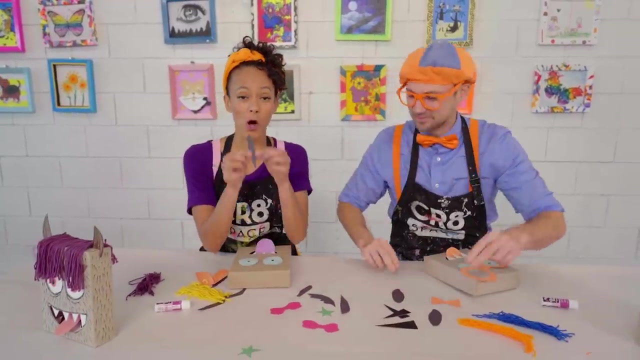 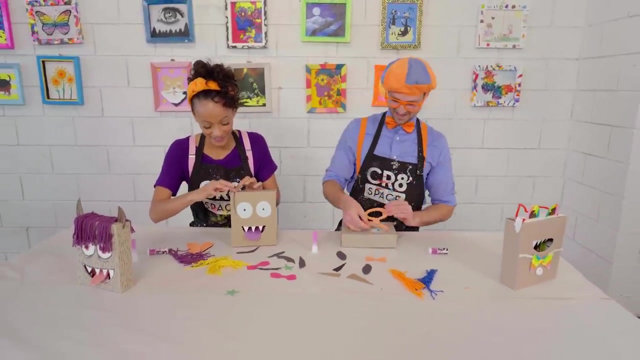 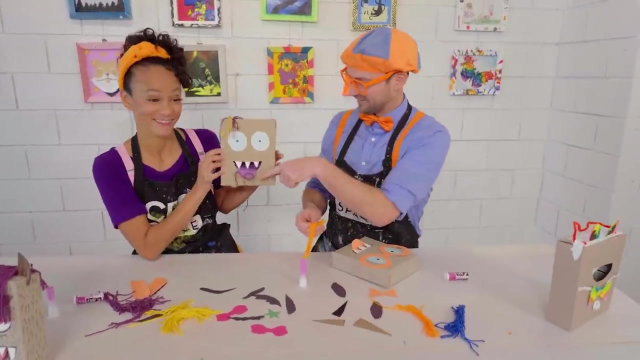 perfect, okay, let's see what we have. oh, look, a pink bow tie if you want to pee. oh yeah, it looks like a really big, uh, eyebrow. yeah, how do i look? oh, very funny, but this could be a very long silly nose. whoa, now, that is silly, yeah, okay. 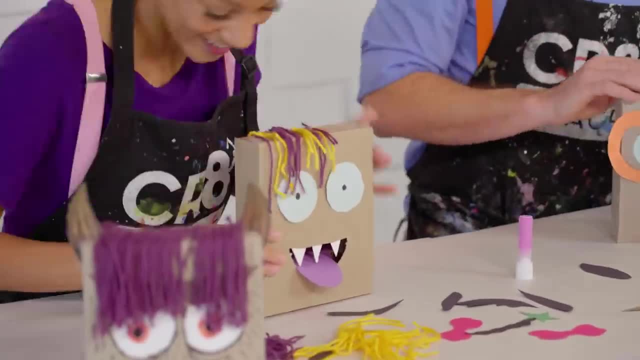 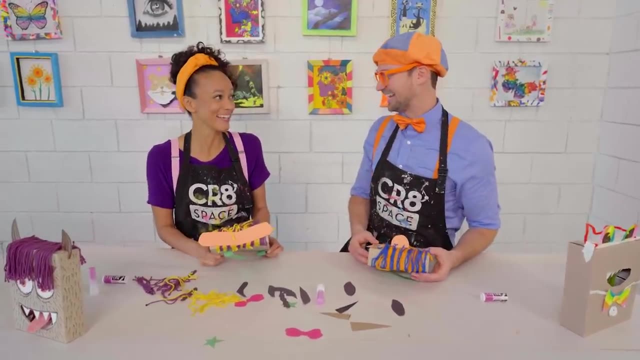 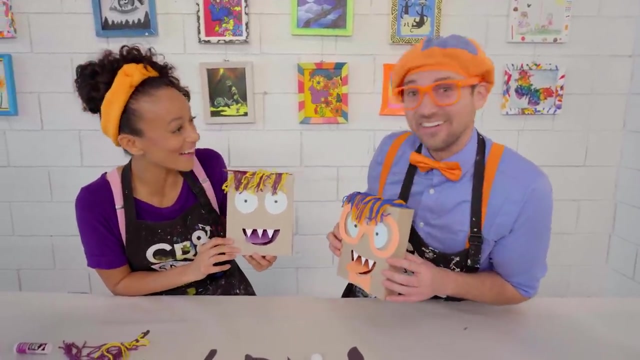 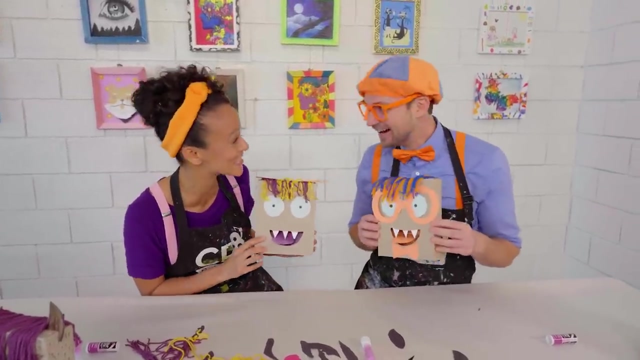 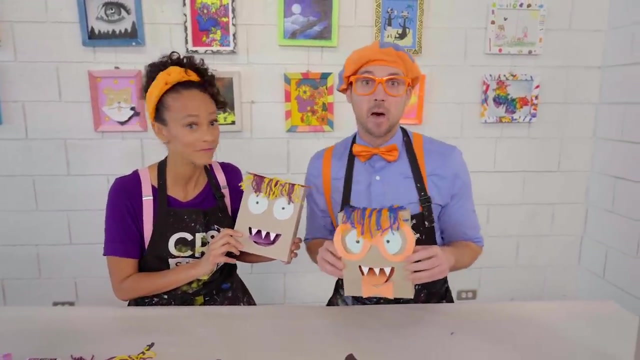 so, oh, all, right, are you ready? yes, i'm so excited to see your monster. here we go. wow, it looks just like you, mika. thank you, monster mika, yours flippy, that looks amazing. oh, thank you, hello, so silly. well, shall we have a monster box puppet show? yes, we shall. yeah. 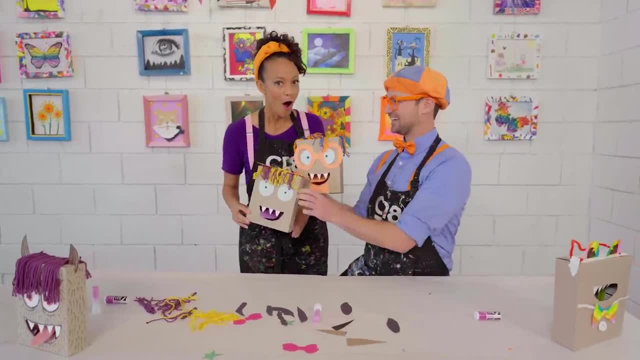 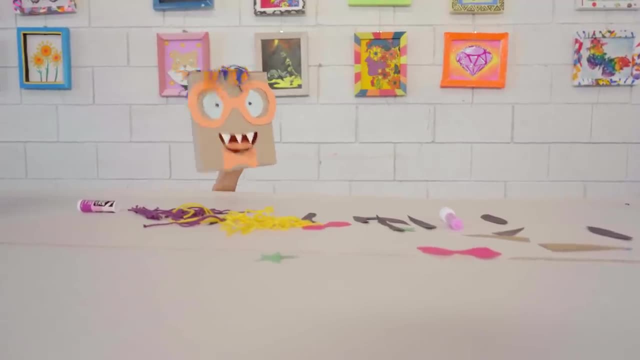 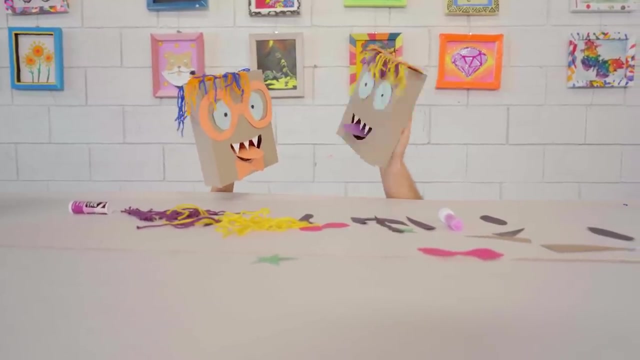 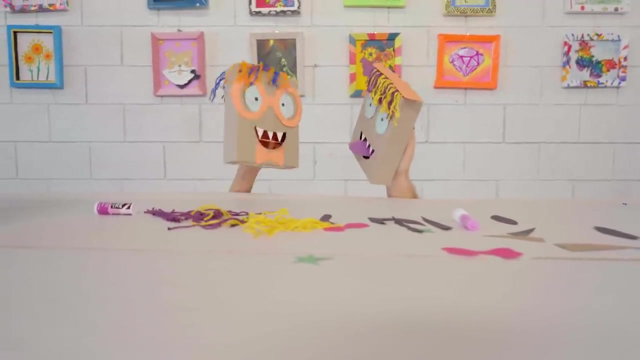 hey, i have an idea though: switch, oh yeah, it's gonna be fun. hello, i'm monster blippy. hello, wow, hey, blippy. oh, i mean monster blippy. you look fabulous. that's right, i'm a silly monster looking good, mika. oh, thank you so much. 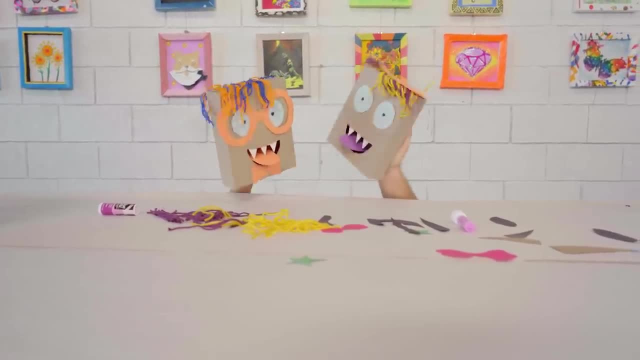 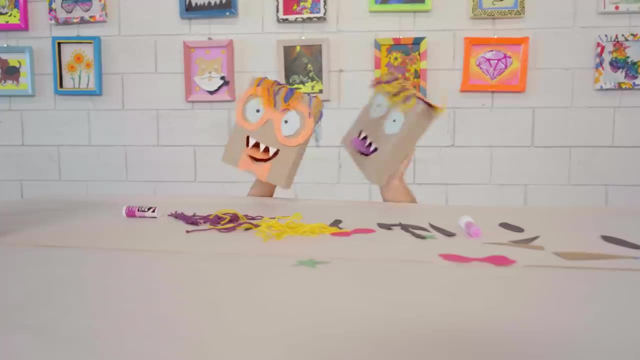 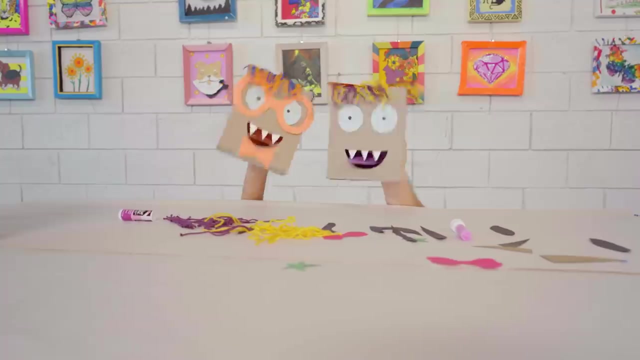 oh, did you notice my purple and yellow hair? of course i did. it does look fabulous. you are so silly, blimpy. that's why you're my best friend. now you're my best friend. oh, no, you're my best friend. oh, mika monster, we have fun together. 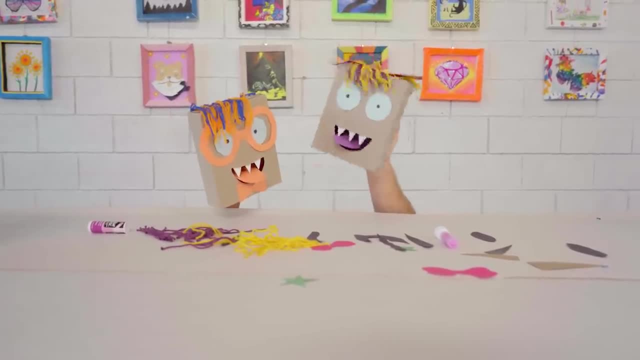 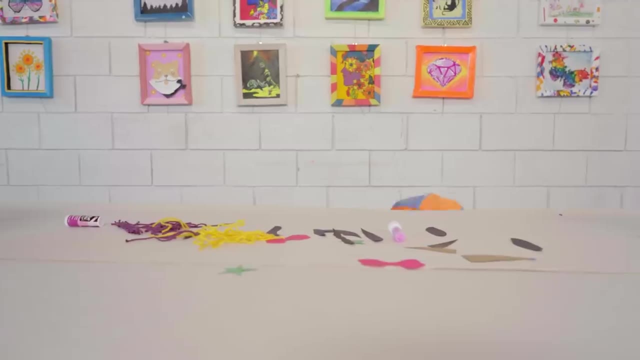 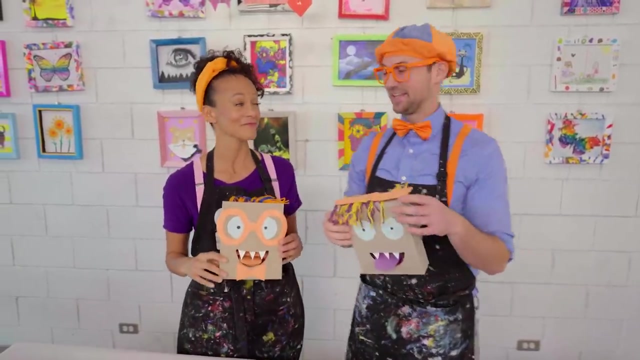 yeah, we do. we go on such fun adventures. that's right. hey, let's go on another one. oh, wow, that was awesome, mika. oh, it's so funny. yeah, and that was really fun making these monster boxes together. yeah, we made a lot of cool things today. we made that really beautiful. 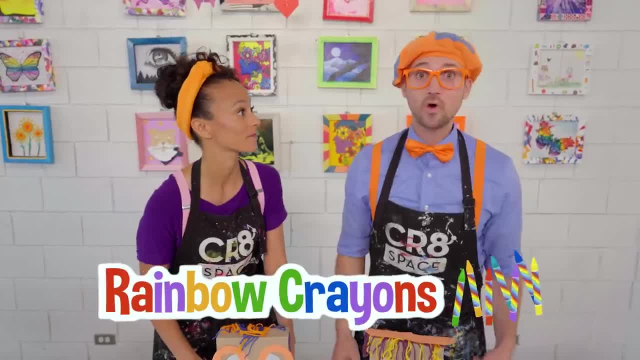 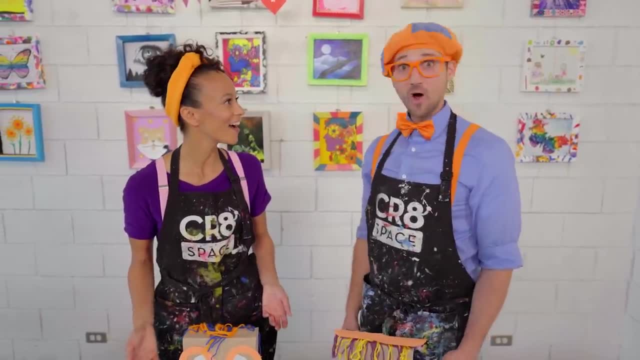 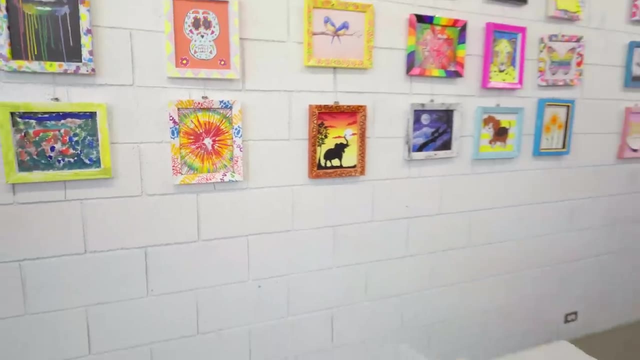 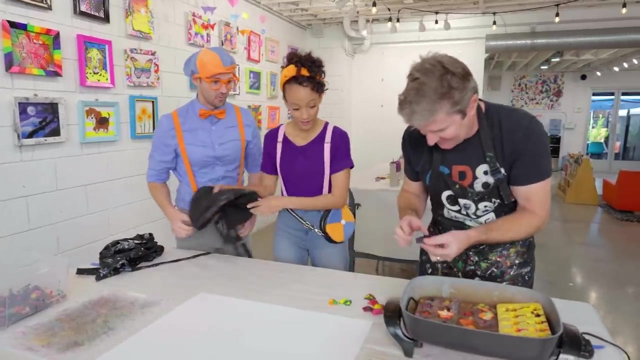 painting together on the canvas. yeah, and those rainbow crayons- wow, i bet they're gonna be so colorful, i know, hey, oh yeah, do you think they're finished yet? i don't know. let's go check them out. wow, oh, hey, hi, welcome back. oh, are they done? they are done. you want to see them wow. 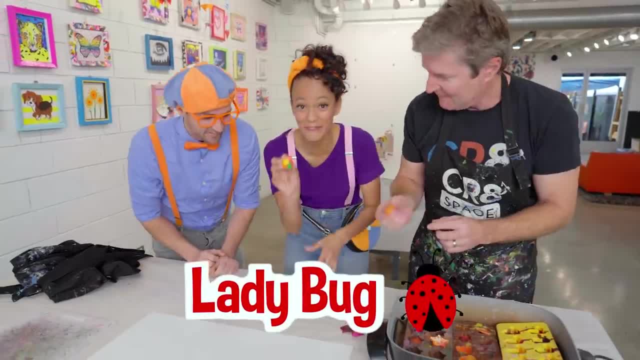 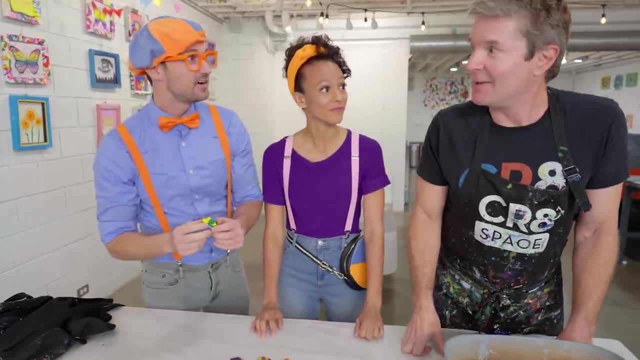 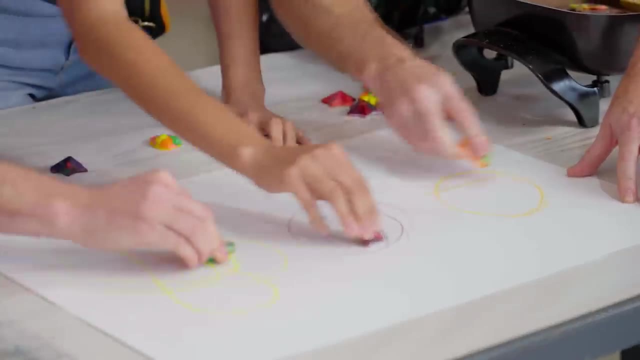 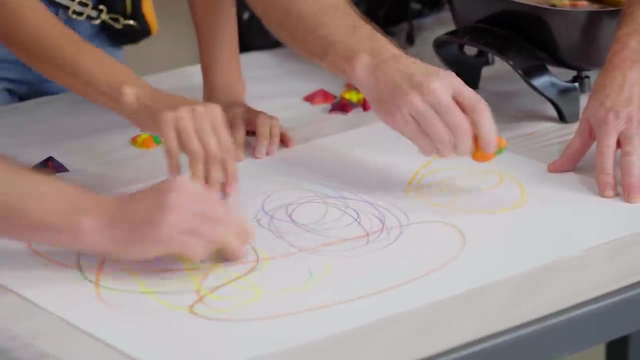 check it out. a star- isn't that cool ladybug, so cute and so colorful. yeah, they look great. wow, you guys want to try them out? yeah, yeah, here, follow me ready, all right, whoa, whoa, whoa. they do change colors when you use them. oh look, i can see blue and purple in mine. wow, that fun mine. 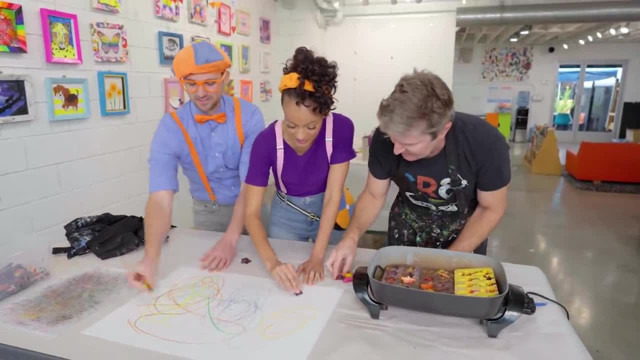 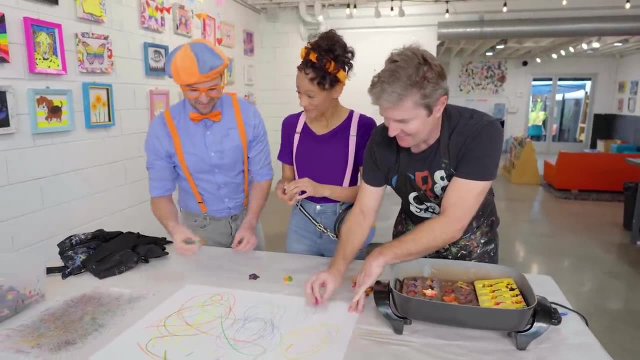 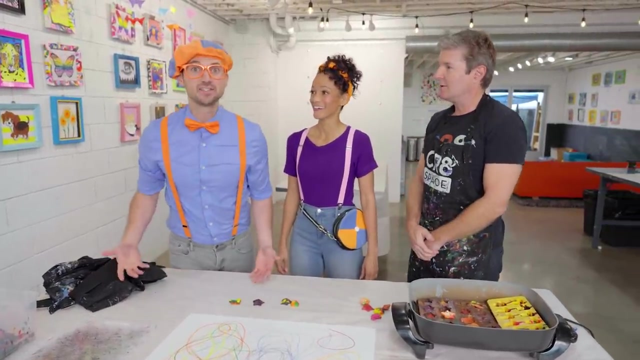 went from yellow to green to orange. oh, i can see yellow in my mouth too. i love what you guys are doing. that looks fantastic. that was so much fun making art today. yeah. what else did you guys do at the studio? oh well, we made some really cool monster boxes, yeah, and we painted a canvas together. 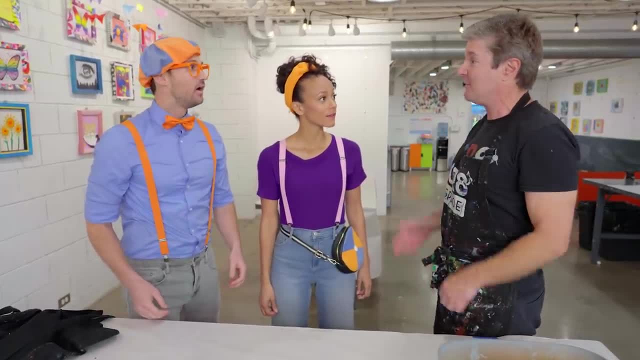 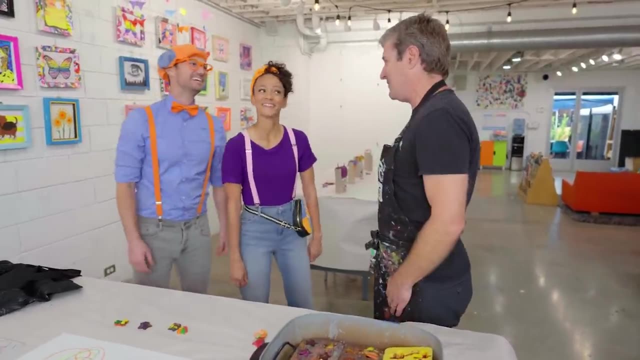 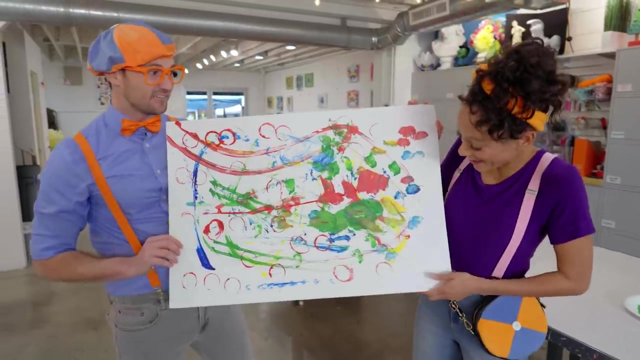 yeah, well, i'll go ahead and clean this up if you guys want to go and see if your stuff's ready. oh yeah, maybe it's dry. yeah, all right, thank you so much. thanks for coming in. it was so nice to meet you guys. all right, see you again. bye, wow, oh, look at me. look, it is dry. yeah, it looks really nice. 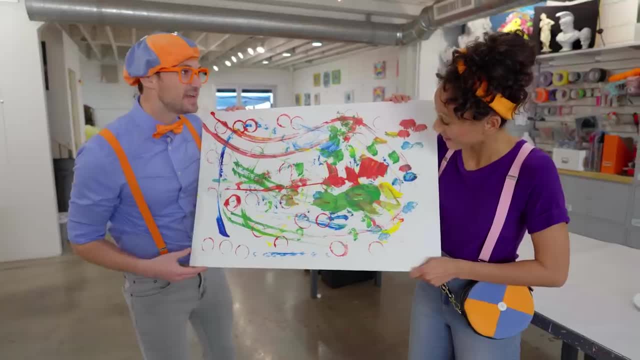 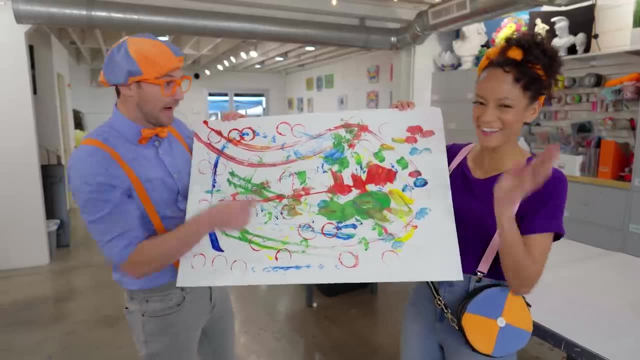 oh yeah, i love the green and the tire tracks that you made. yeah, and here are the circles that we made with paper tubes. oh yeah, and you can't forget about my piece of tape. wow, should we go hang it up? yeah, let's do it all right. 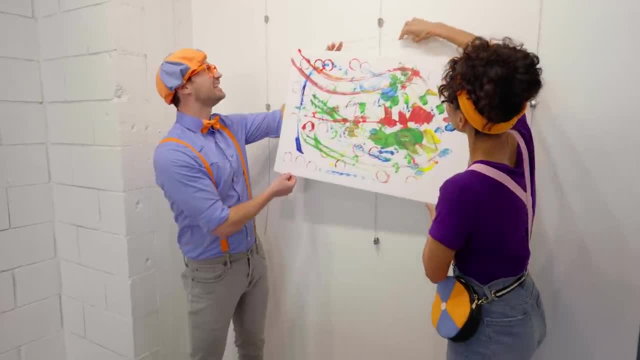 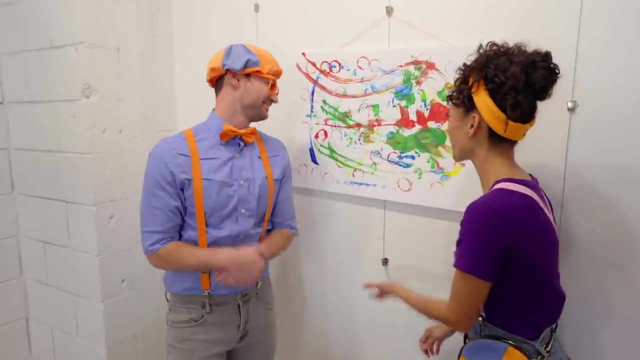 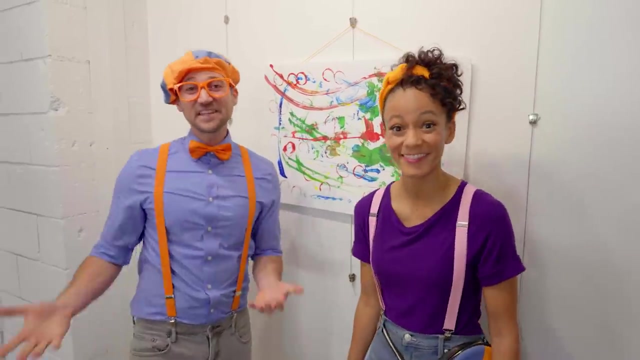 now everyone can see it. yeah, here we go. what a beautiful masterpiece. yeah, i really love all of the colors that we used and that we made it together. yeah, we did such a great job. yeah, i think so too. well, this is the end of this video, but if you want to watch more of my videos, all you have to do is search for my name. 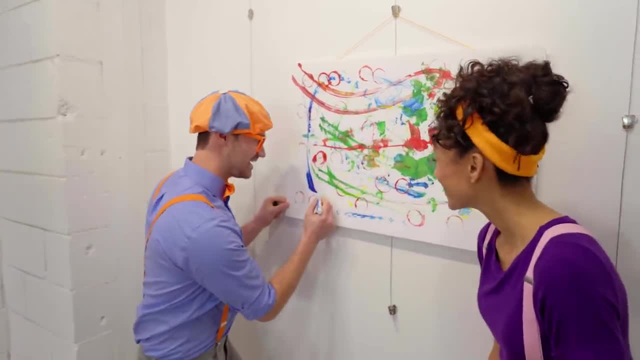 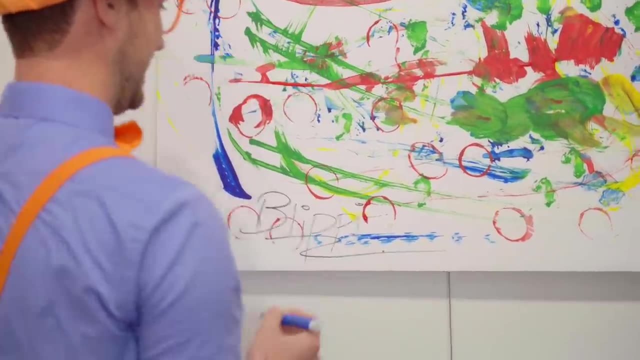 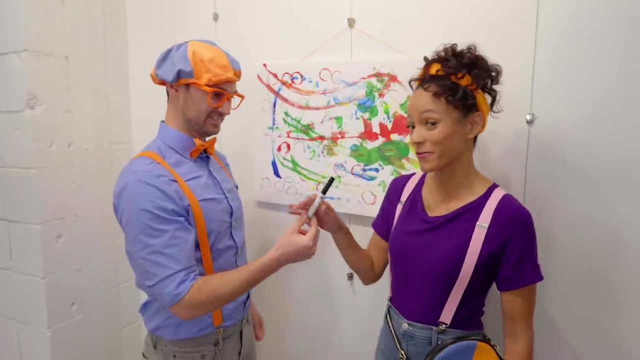 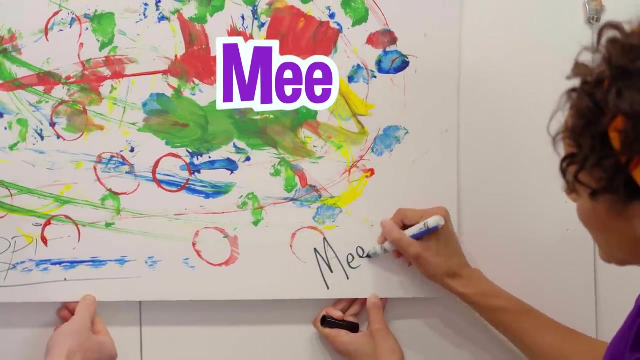 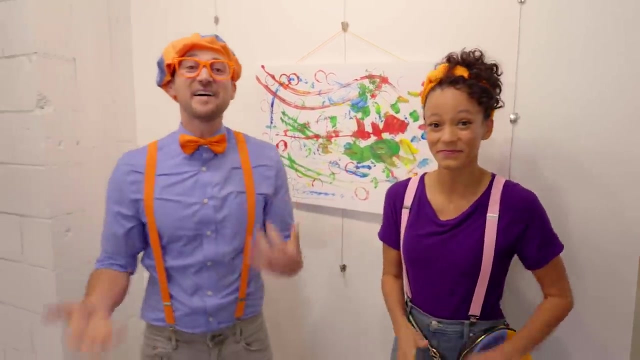 you spell my name with me? yeah, ready, yeah, b l, i, p, p, i blippy, and if you want to search for me, you can spell my name: mika. will you spell my name with me? awesome, m e, e, k a, h, Mika. Oh, what a fun video. 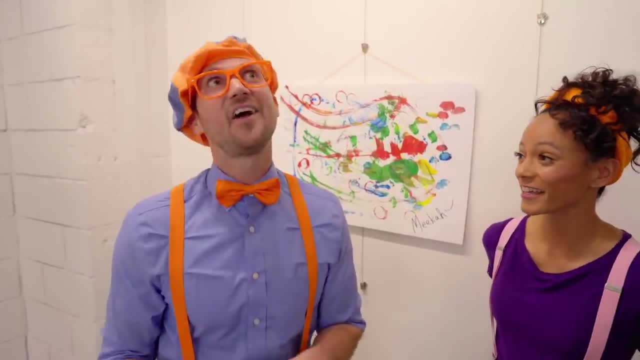 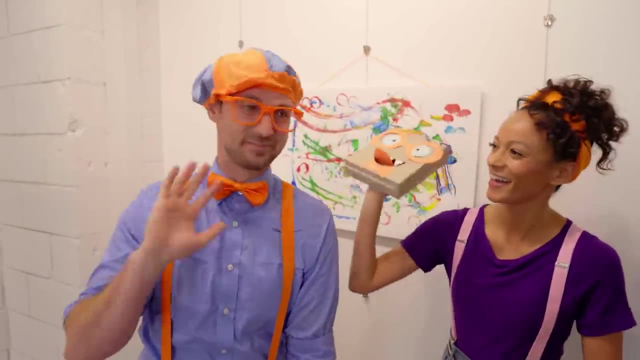 And it was so much fun making art today together. Art is so much fun because it's also unique. I love art too. Blippi, Whoa, Hey, Monster Box, Blippi, Hello, Hello, All right, See you again. 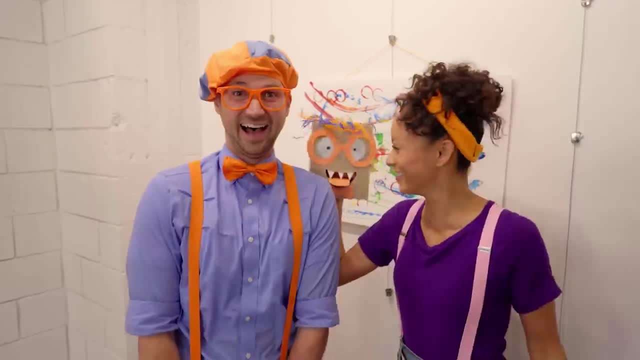 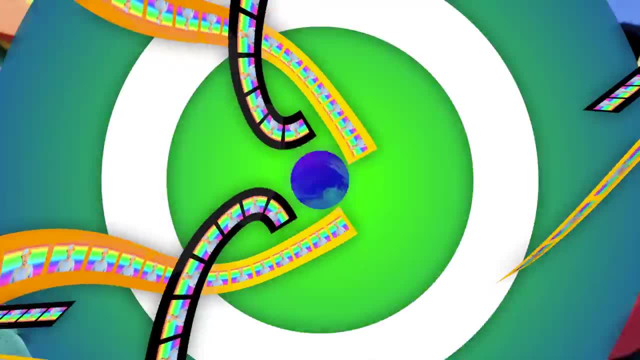 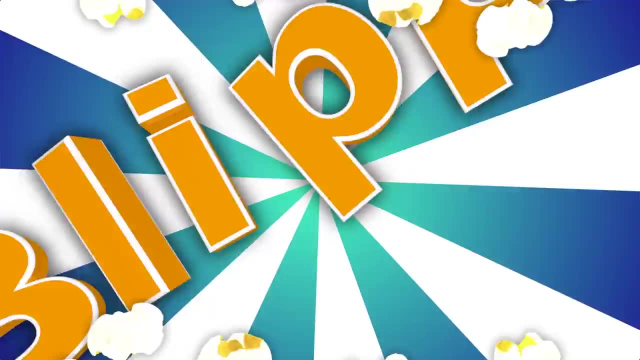